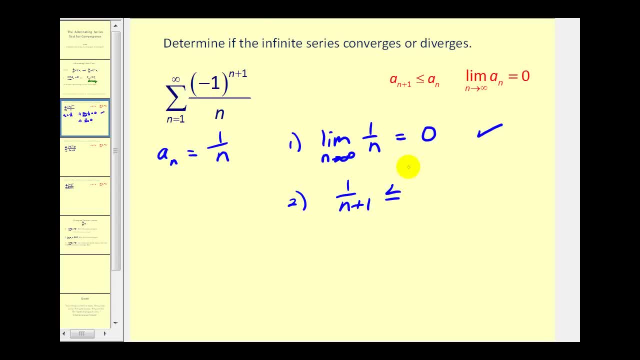 And that must be less than or equal to a sub n, which is just one over n. Looking at this, we can tell that this fraction has larger denominators and therefore would always be less than or equal to one over n. So these two conditions are met. 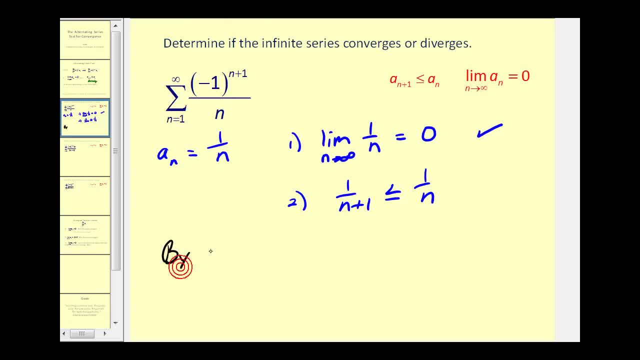 So by the alternating series test, the given series converges. So this is kind of interesting, because the harmonic series diverges, but the alternating series ends somewhere. harmonic series converges based upon this test. Let's take a look at another alternating series. 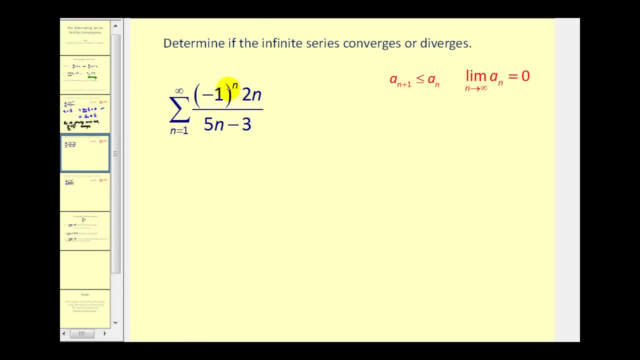 Again. our first step is to identify a sub n, which is a non-alternating part of this formula. So a sub n is going to equal two n divided by five n minus 3.. This limit has to be equal to zero before we can proceed. 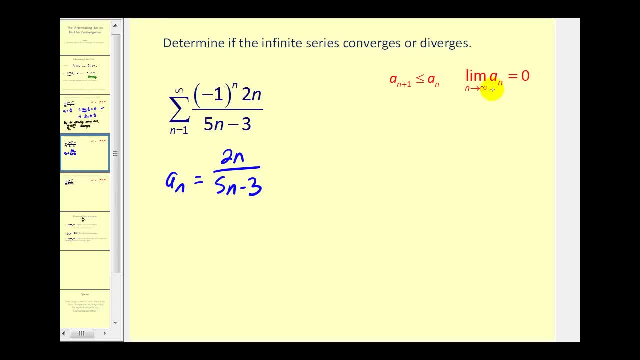 with the alternating series test. And it's not Notice, the degree of the numerator and denominator are the same. so this limit is equal to the ratio of the leading coefficients, which is two-fifths. So this doesn't equal zero. so it's going to be. 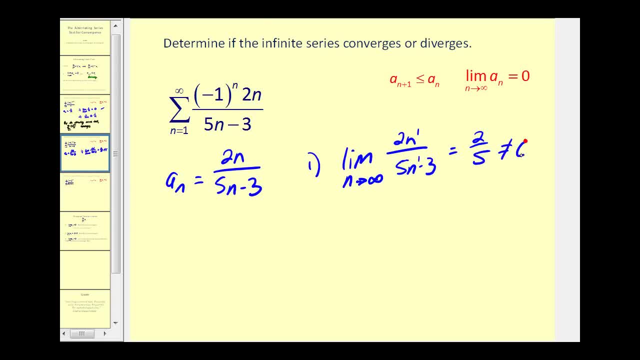 two-fifths of the number of the leading coefficients. So that's two-fifths. So it fails the alternating series test. So not only is this limit not equal to zero, it fails the nth term divergent test. So this alternating series diverges. 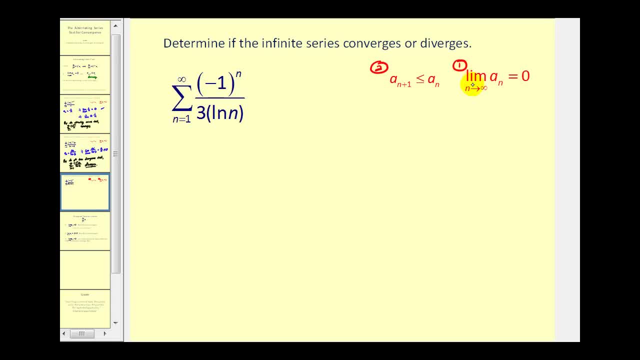 Let's take a look at one more. So first we'll check to see to make sure this limit is equal to zero And then we'll check to see if the non-alternating series is decreasing. So a sub n is going to equal 1 over 3 times natural log n.